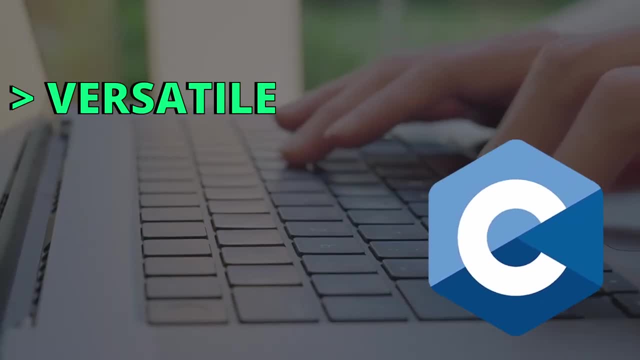 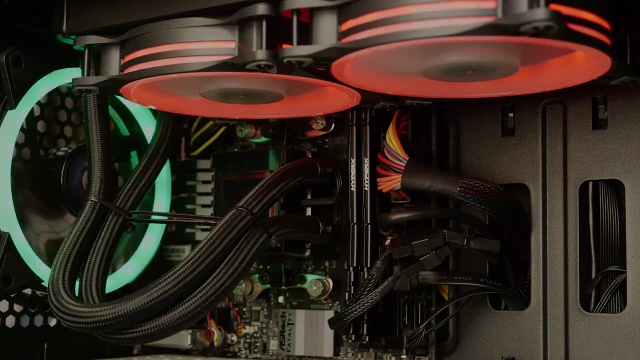 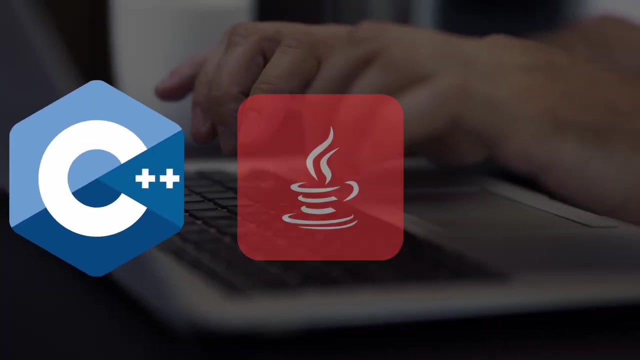 The C programming language, created by Dennis Ritchie, is a versatile and powerful language known for its efficiency and flexibility. It provides low-level access to memory, making it ideal for applications that require interaction with hardware. ANSI is known to be the mother of all languages, like C++, Java and Python. 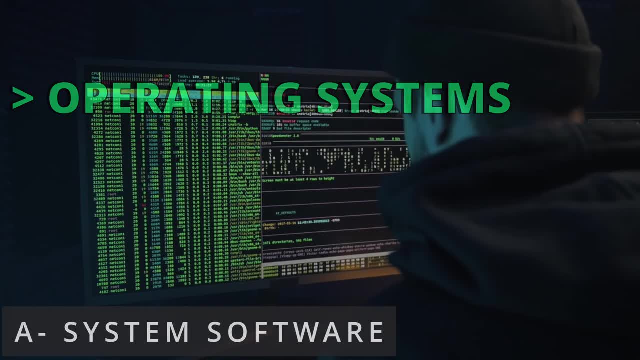 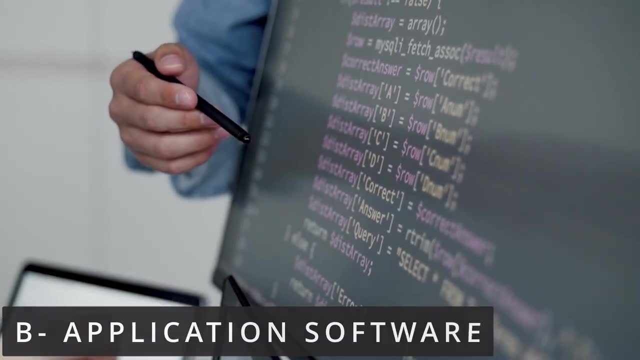 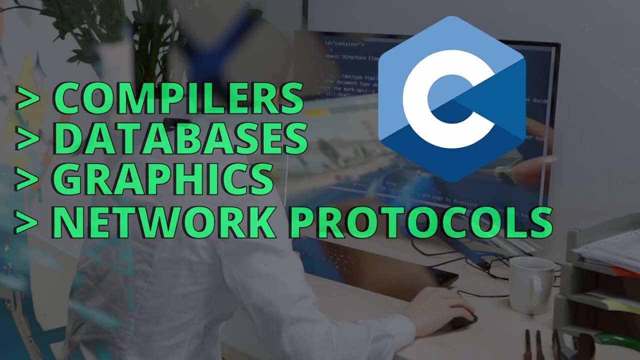 The C programming language can be used to build system software like operating systems, device drivers, firmware and embedded systems. Applications that require efficiency and high performance are written in C. Applications like compilers, databases, graphics and network protocols are written in C. Also, C is used to develop games due to its efficiency and 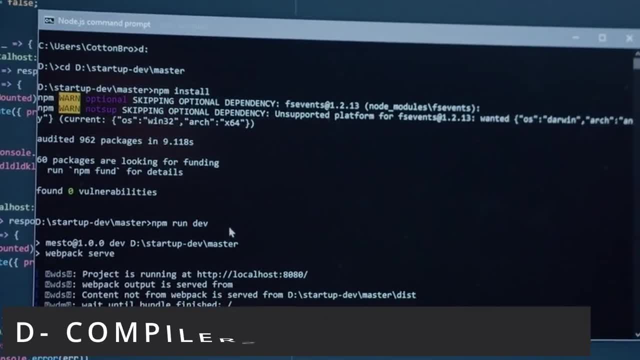 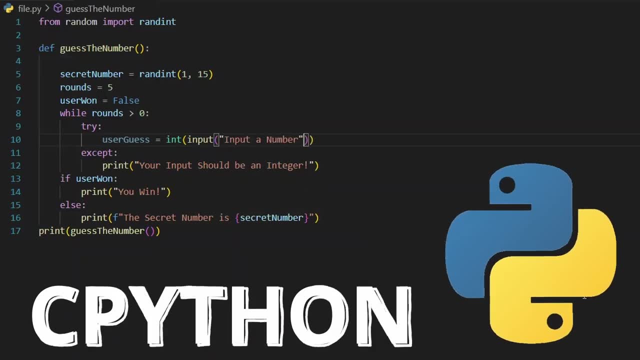 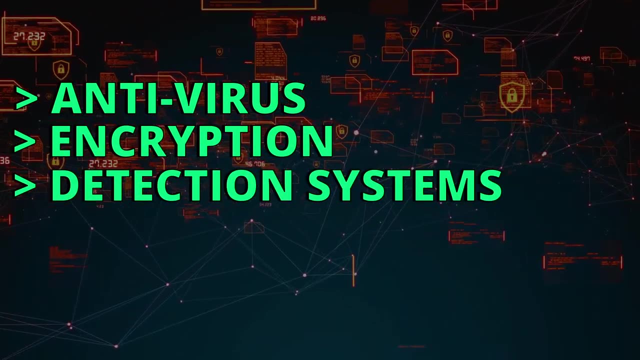 ability to interact with hardware. As mentioned, C is used to build compilers and interpreters for other languages, like the Python interpreter called CPython is implemented in C. for example, Security tools are built using C. Tools like antivirus, encryption algorithms, detection systems are built using C. 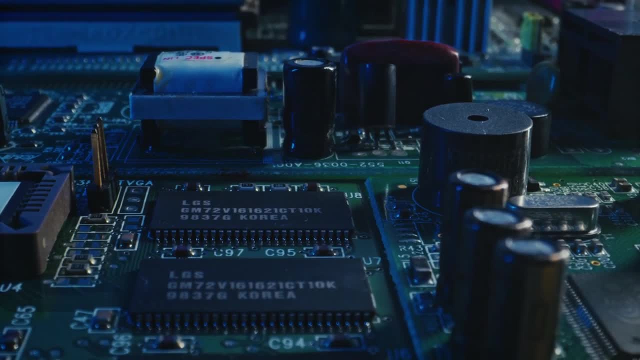 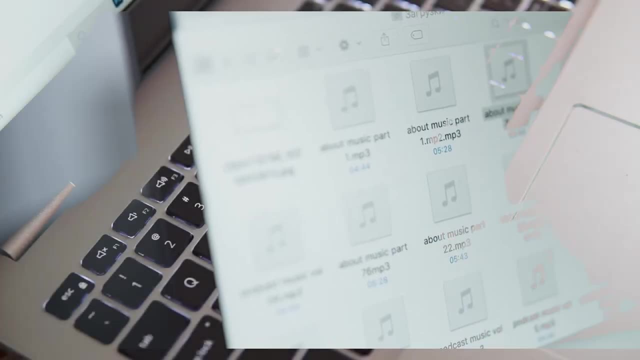 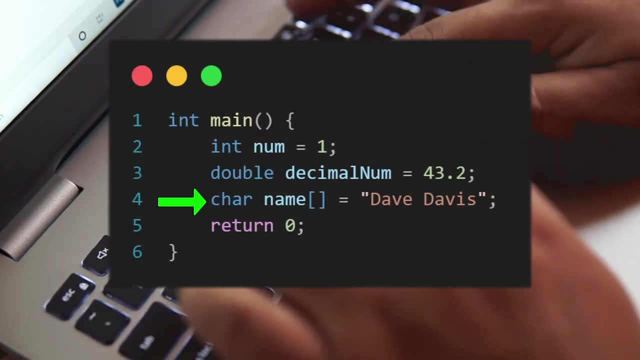 Due to its ability to manipulate low-level data and hardware interaction. C is a compiled language, meaning its source code is directly converted by the compiler to an executable file. C is also a statically typed language, meaning the programmer must specify the type of data the variable will store beforehand. 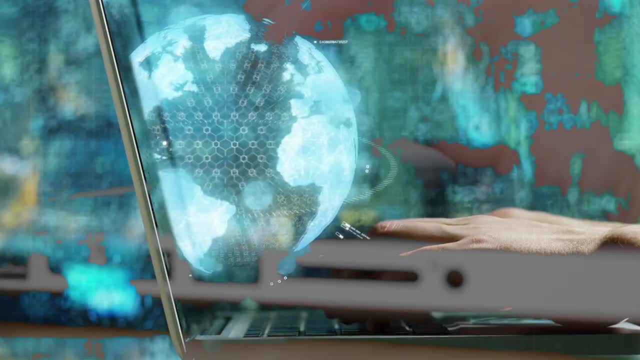 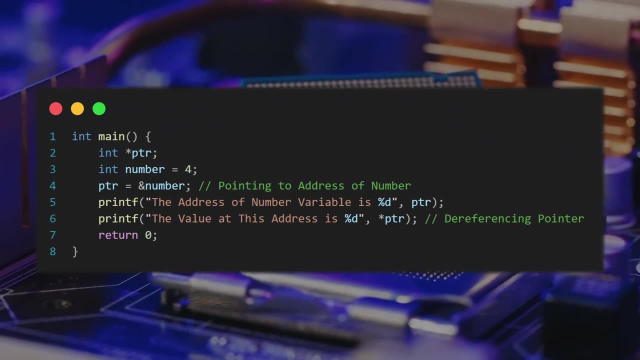 unlike dynamic typing which is guessed during runtime. One way of accessing memory in C is with pointers which points to a certain value inside memory. Like this, you can directly access and change the original memory in C. You can also access the original memory in C. 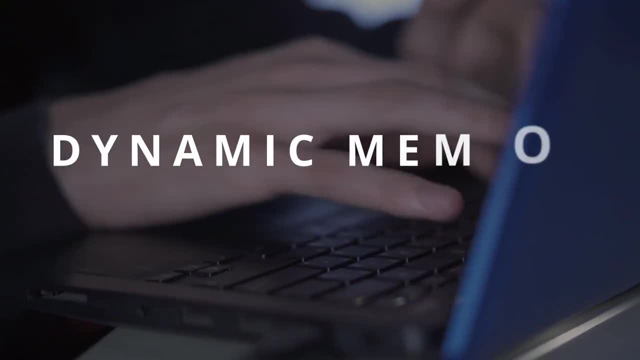 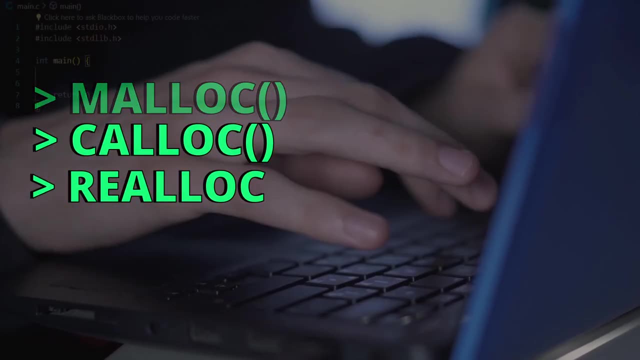 which is the original value in memory. Also, with the help of dynamic memory allocation, you can allocate and deallocate space in the heap using functions like malloc, calloc or realloc. Both malloc and calloc are used for dynamic memory allocation. like here, we are creating a dynamic 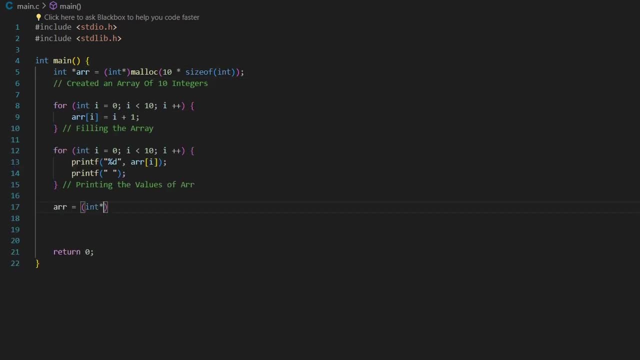 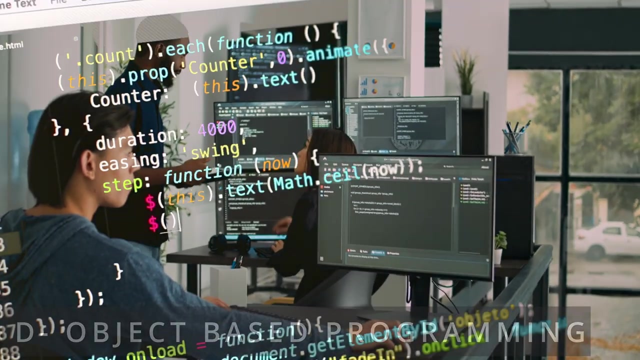 array of 10 integers using malloc. Also, we use realloc to allocate or resize our array to add 10 more integers. At the end of your program you should always deallocate the space created with the free function. The C programming language lacks object-oriented programming, However. 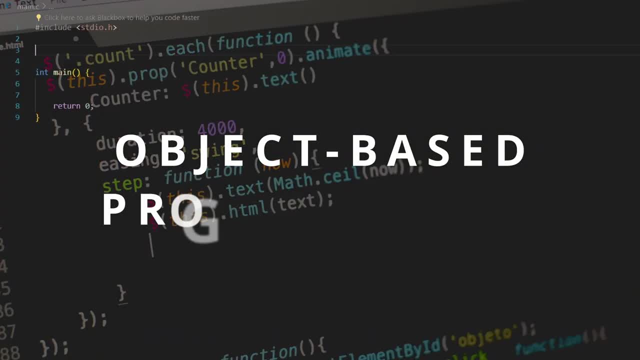 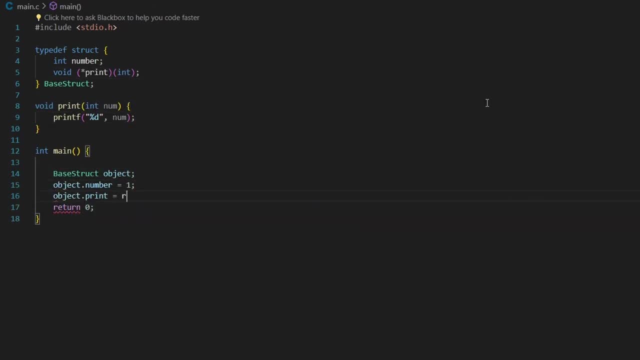 C does support object-based programming principles where you create a structure that has data, members and function pointers, which you can create an object of this structure and use its members in the main function, The C++ language, which is a successor of the C language.